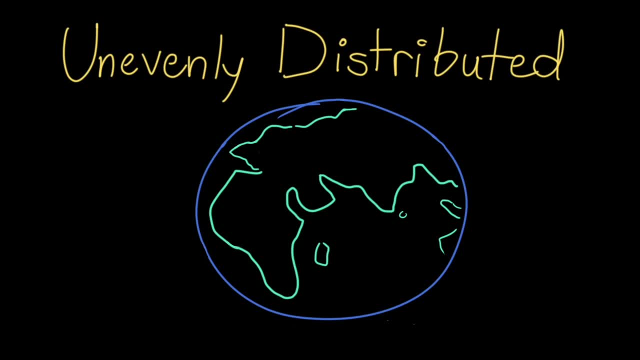 such as plate tectonics, that take place in specific locations on Earth. As a result, non-renewable resources like soil, minerals and fossil fuels are often concentrated in the places where they first formed. Let's take a look at one type of non-renewable resource. 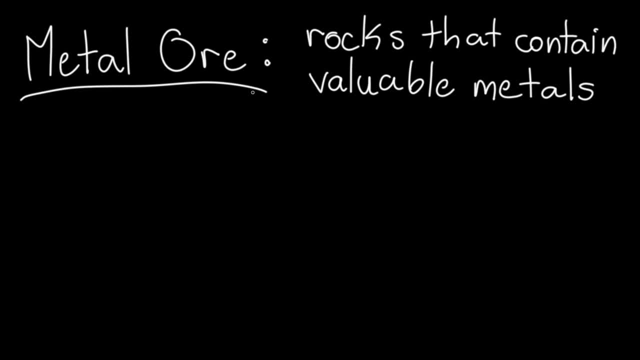 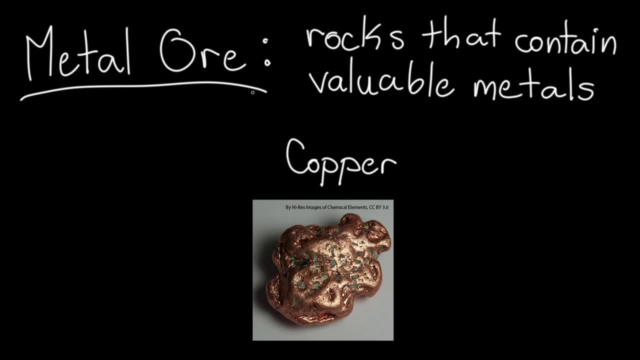 metal ore. Metal ores are rocks that contain valuable metals that people can extract, and they're often found in large accumulations called deposits. For example, most copper ore is found in what are called porphyry copper deposits. Porphyry just means that the rock. 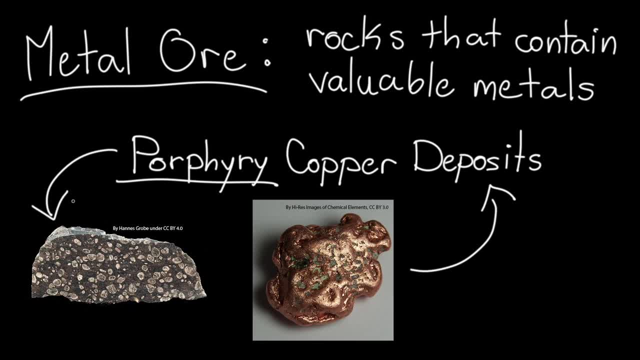 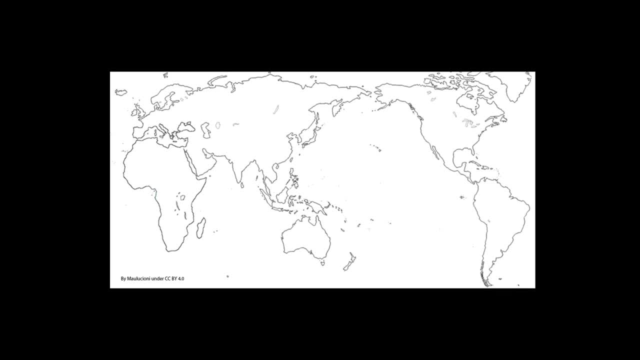 that makes up these deposits contains a mix of large and small crystals, like in this image here. Porphyry, copper deposits form in subduction zones along convergent tectonic plate boundaries. Today, most subduction zones are found along Pacific coastlines, so you can expect to find 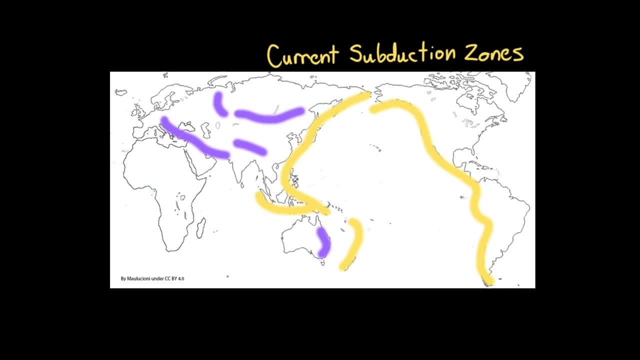 a lot of porphyry copper deposits, But if you're not sure, you can find a lot of porphyry copper mines in these places. However, we also find many of these ore deposits throughout Eurasia and Australia. Why, Turns out, many of these places were subduction zones in the ancient past. 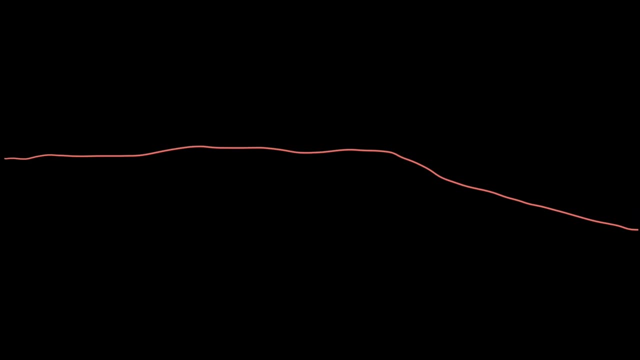 The geologic processes that form non-renewable resources are always happening, even if they occur over thousands or millions of years. This means that non-renewable resources are not always found where they first formed. Porphyry copper deposits follow the same slow life cycle as many. 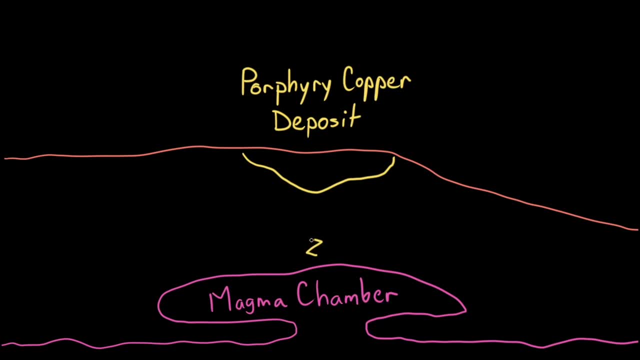 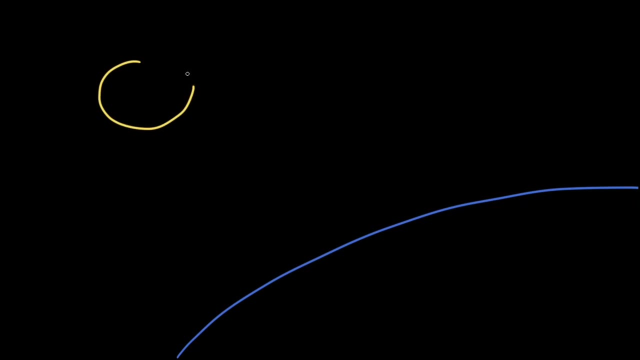 other metal ores, forming in magma chambers below the crust, then uplifting towards the surface through tectonic activity. Once exposed to the elements, the deposits can experience weathering and erosion, which allows them to gradually recycle back into the Earth, Unless people find and mine them first. How can renewable natural resources be unevenly? 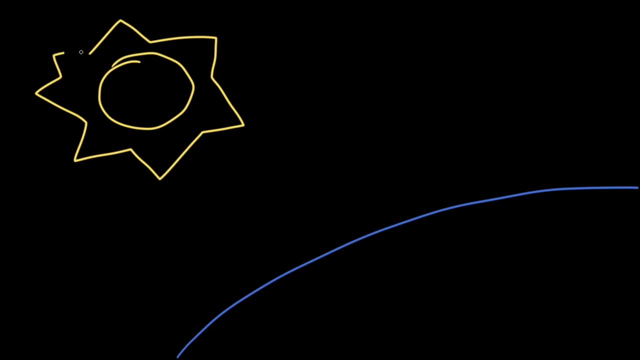 distributed across Earth, though Doesn't everywhere have things like sunlight and wind. Well, yes, but Earth's tilt means that some places experience more direct sunlight throughout the year than others, And geography and other factors mean that some places are windier than others. 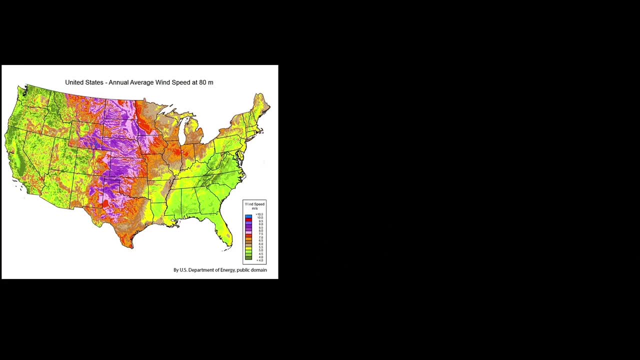 For example, take a look at this map of average annual wind speeds across the contiguous United States. These purple, red and orange places typically experience higher wind speeds, while these green and yellow places typically experience lower wind speeds. As a result, this central part of the country here has a much higher